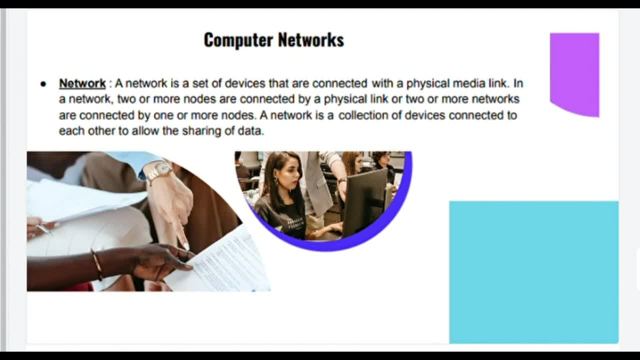 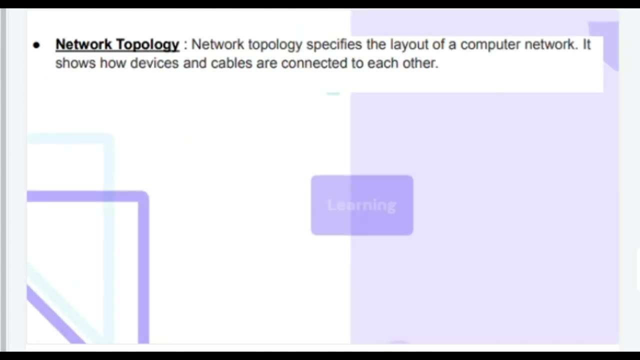 In a network, two or more nodes are connected by a physical link, or two or more networks are connected by one or more nodes. A network is a collection of devices connected to each other to allow the sharing of data. Network topology. Network topology specifies the layout. 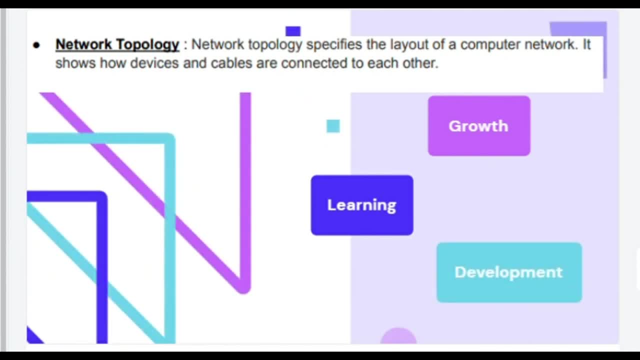 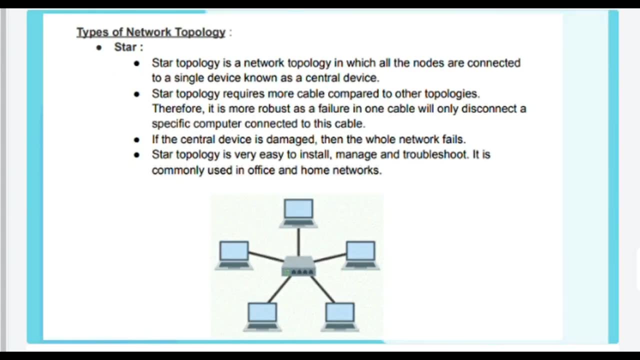 of a computer network. It shows how devices and cables are connected to each other. Types of network topology: Star Star topology is a network topology in which all the nodes are connected to a single device known as a central device. Star topology requires more. 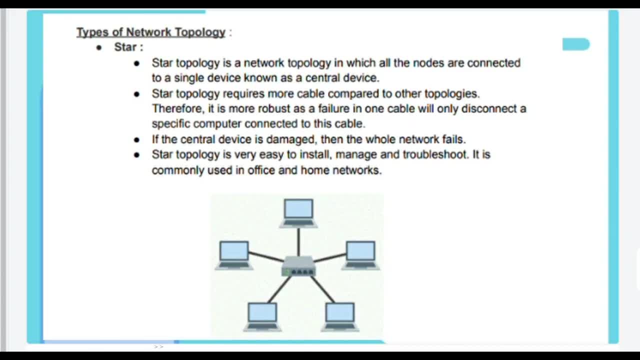 cable compared to other topologies. Therefore it is more robust, as a failure in one cable will only disconnect a specific computer connected to this cable. If the central device is damaged, then the whole network fails. Star topology is very easy to install, manage and troubleshoot. It is. 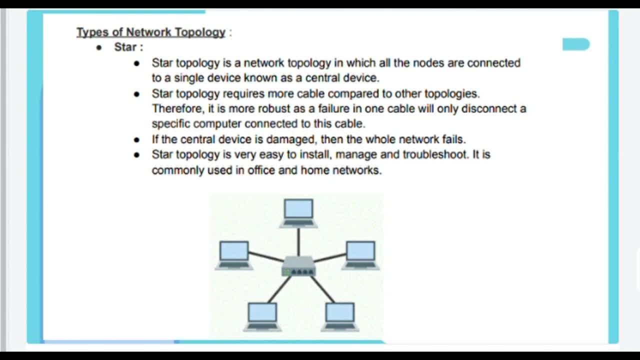 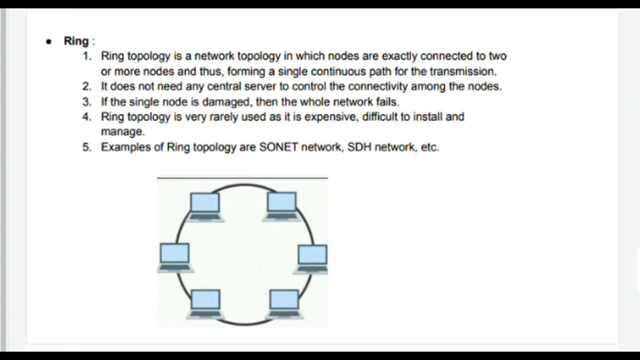 commonly used in office and home networks. Ring One. ring topology is a network topology in which nodes are exactly connected to two or more nodes and thus forming a single continuous path for the transmission. Two, it does not need any central server to control the connectivity among the nodes. Three, if the single node is damaged, 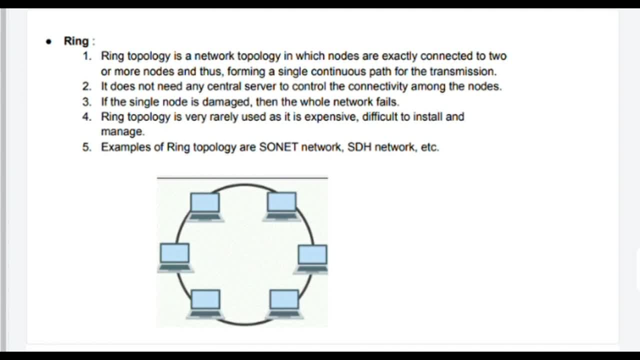 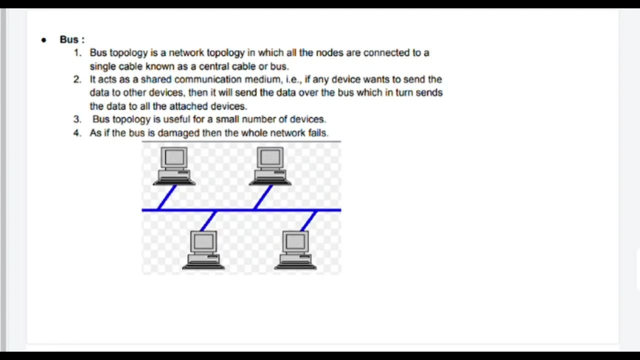 then the whole network fails. Four: ring topology is very rarely used as it is expensive, difficult to install and manage. Five examples of ring topology are Sonet network, SDH network, etc. Bus One bus topology is a network topology in which a network is connected to a single. 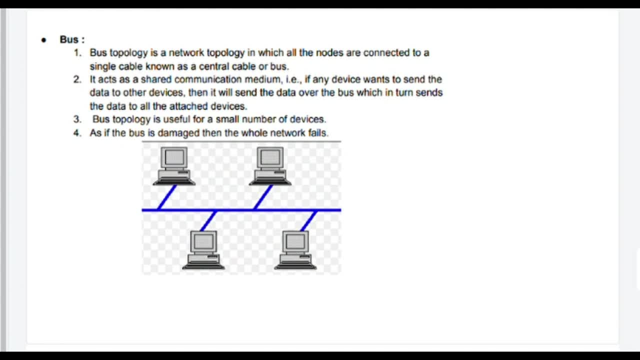 in which all the nodes are connected to a single cable, known as a central cable or bus 2.. It acts as a shared communication medium, ie if any device wants to send the data to other devices, then it will send the data over the bus, which in turn sends the data to all the 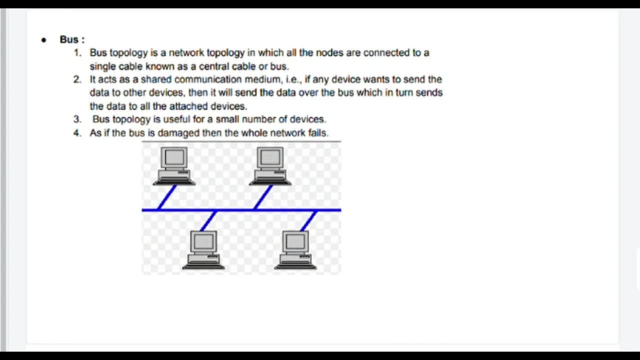 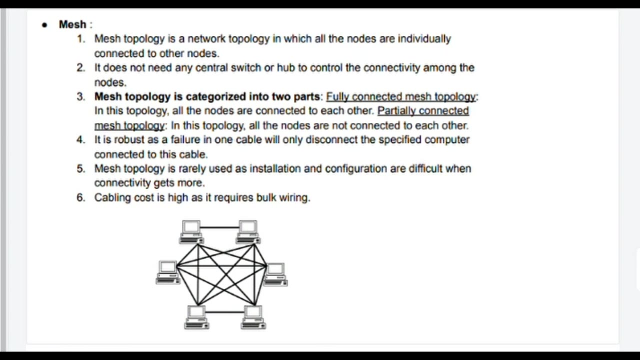 attached devices. 3. Bus topology is useful for a small number of devices. 4. As if the bus is damaged, then the whole network fails. Mesh 1. Mesh topology is a network topology in which all the nodes are individually connected to other nodes. 2. It does not need any central.